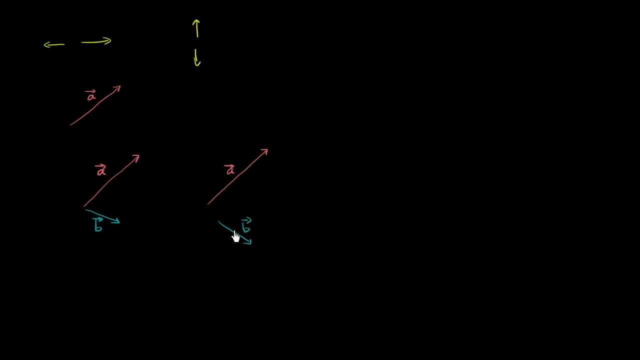 I could draw vector b. I could draw vector b over here. It's still vector b. It still has the same magnitude and the direction. Notice, we're not saying that its tail has to start at the same place that vector a's tail starts at. 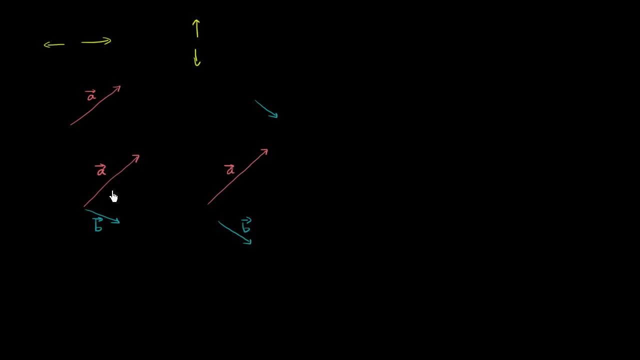 I could draw vector b over here. I could always have the same vector, but I can shift it around So I could move it up there As long as it has the same magnitude, the same length and the same direction. And the whole reason I'm doing that is because the way to visually add vectors 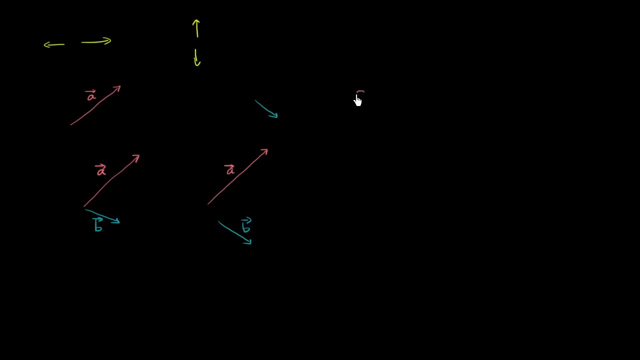 If I wanted to add vector a plus vector b- and I'll show you how to do it more analytically in a future video- I could literally draw vector a. I draw vector a, I put vector a right over there And then I can draw vector b, but I put the tail of vector b to the head of vector a. 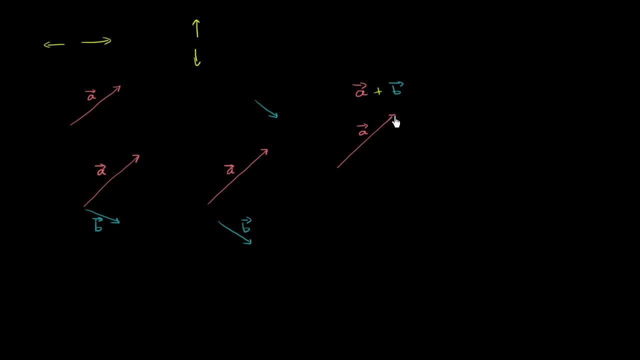 So I shift vector b over, so its tail is right at the head of vector a, And then vector b would look something like this: It would look something like this: And then, if you go from the tail of a all the way to the head of b, 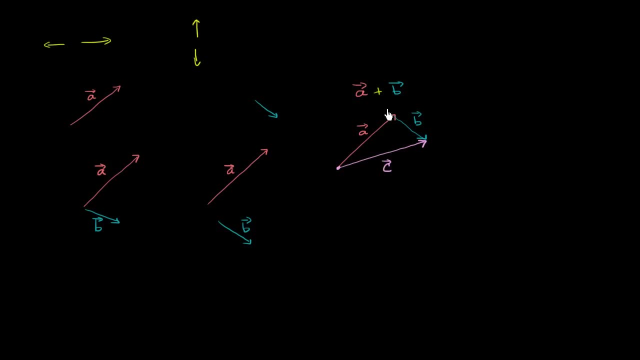 and you call that vector c. and you call that vector c. that is the sum of a and b. That is the sum of a and b And it should make sense If you think about it. let's say these were displacement vectors. 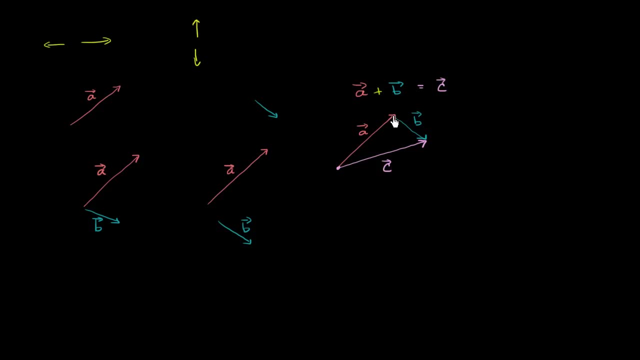 So a shows that you're being displaced this much in this direction. b shows that you're being displaced this much in this direction. So the length of b in that direction And I would say you have a displacement of a and then you have a displacement of b. 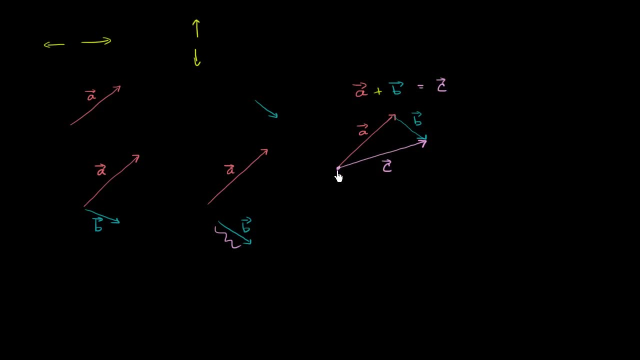 What is your total displacement? So you would have had to be, I guess, shifted this far in this direction And then you would be shifted this far in this direction. So the net amount that you've been shifted is this far in that direction. 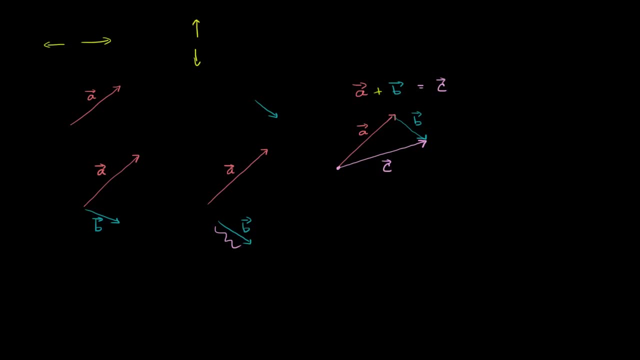 So that's why this would be the sum of those. Now we can use that same idea to break down any vector in two dimensions into its- we could say into its- components, And I'll give you a better sense of what that means in a second. 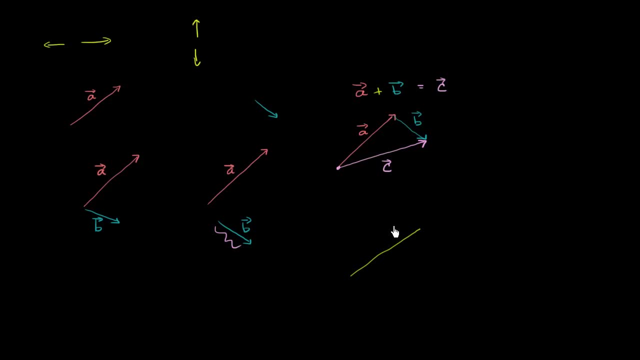 So if I have vector a, let me pick a new letter. Let's call this vector vector x. Let's call this vector x. I can say that vector x is going to be the sum of, is going to be the sum of this vector right here in green. 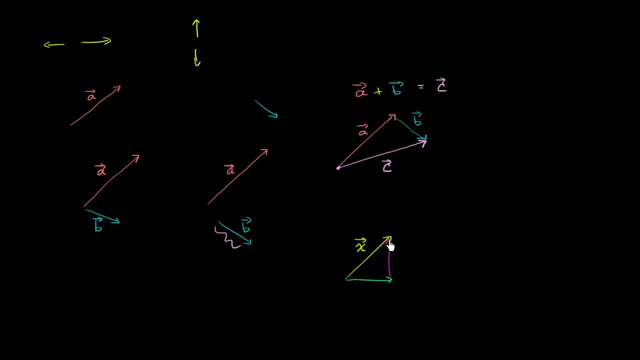 and this vector right here in red, Notice, if I take, if I x starts at the tail of the green vector and goes all the way to the head of the magenta vector And the magenta vector starts at the head of the green vector. 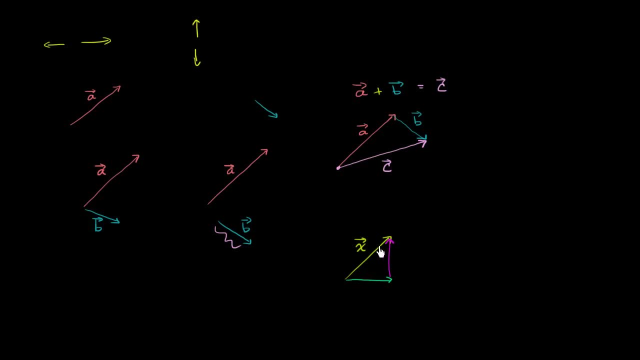 and then, and then finishes. I guess, well, where it finishes is where vector x finishes, And the reason why I do this- and you know this hopefully from this explanation right here- says: okay, look, vector green. 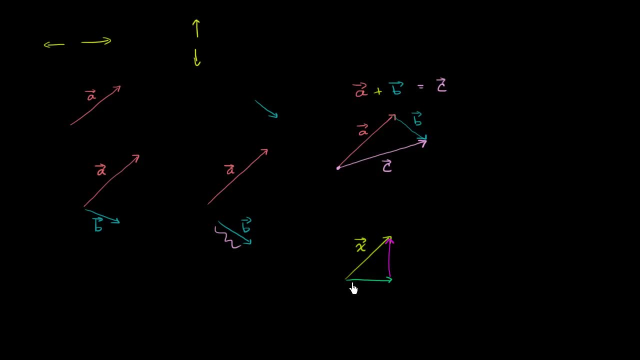 the green vector plus the magenta vector gives us this x vector. That should make sense. I put the. I put the head of the green vector to the tail of this magenta vector right over here. But the whole reason why I did this is: 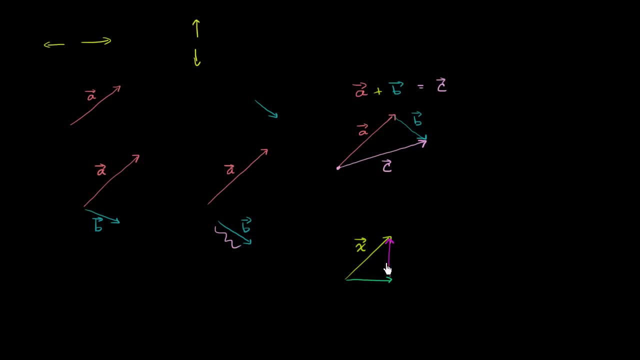 if I can express x as the sum of these two vectors. it then breaks down x into its vertical component and its horizontal component. So I could call this, I could call this the. I could call this the horizontal component, or I should say the vertical component. 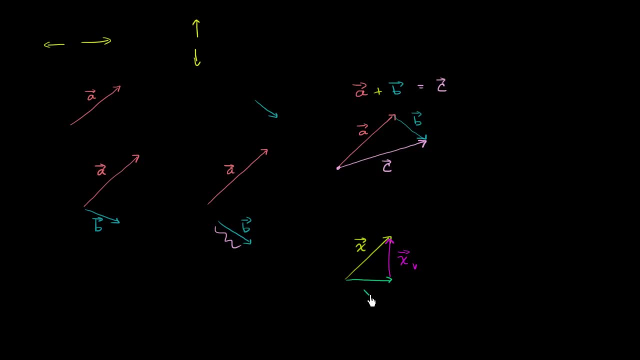 x vertical, and then I could call this over here. I could call this over here the x horizontal, Or another way I could draw it. I could shift this x vertical over. Remember, it doesn't matter where I draw it, as long as it has the same magnitude and direction. 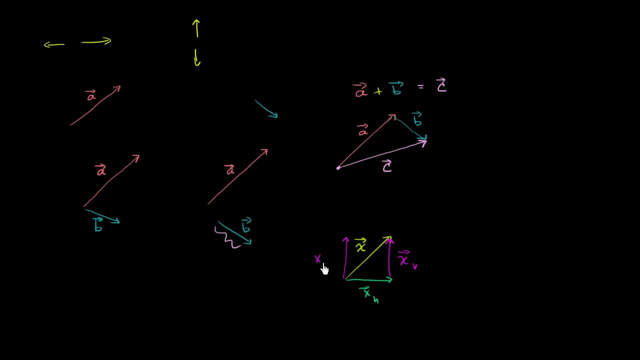 and I could draw it like this: x- vertical. And so what you see is is that you can express this vector x. you can express this vector x- let me do it- the same colors. you can express this vector x as the sum of its horizontal and its vertical components. 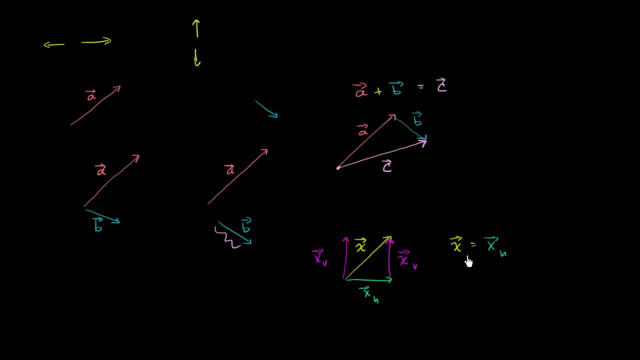 As the sum of its horizontal and its vertical components. And we're going to see over and over again that this is super. this is super powerful because what it can do is it can turn a two-dimensional problem into two separate one-dimensional problems, One acting in a horizontal direction. 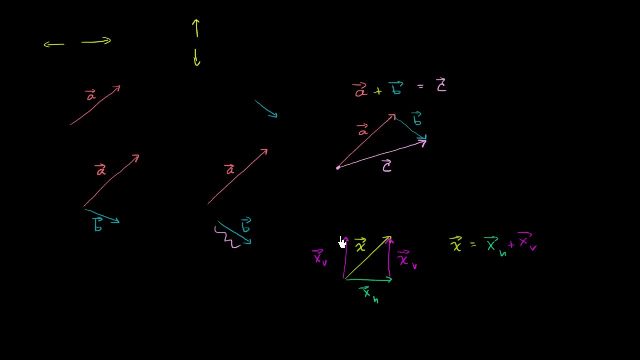 one acting in a vertical direction. one acting in a vertical direction. Now, let's do it a little bit more mathematical. I've just been telling you about length and all of that, but let's actually break down. let me just show you what this means. 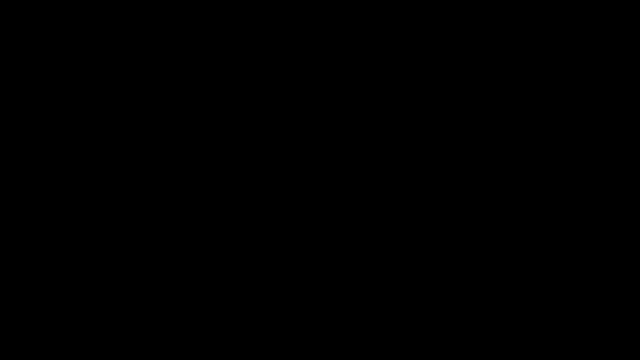 to break down the components of a vector. So let's say: let's say that I have a vector that looks like this. Let me do my best to. so let's say I have a vector that looks like this: Its length is five. 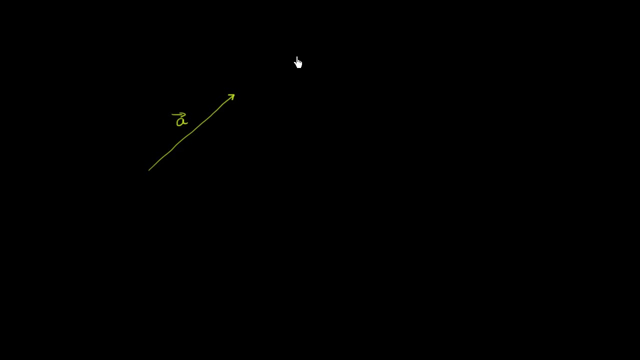 so let me call this vector a, And I will say so. vector a's length is equal to five, And let's say that its direction we're going to give it, we're going to give its direction by the angle between the direction it's pointing at. 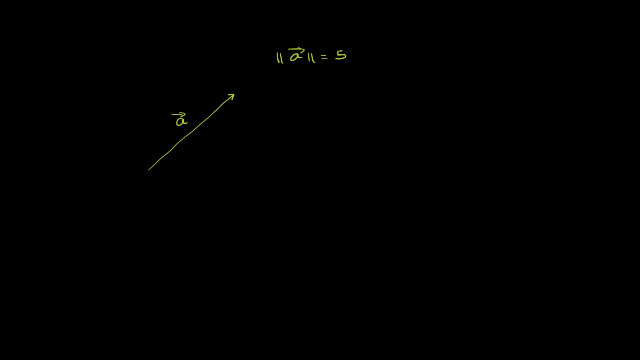 and the positive x-axis. So maybe I'll draw some an axis over here. So let's say that this right over here is the positive y-axis going in the vertical direction, This right over here is the positive x-axis going in the horizontal direction. 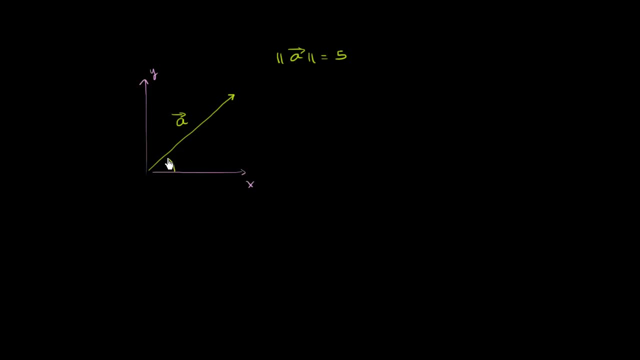 And to specify this vector's direction, I will give this angle right over here, And I'm going to give a very peculiar angle, but I picked this for a specific reason, just so things work out neatly in the end. And I'm going to give it in degrees. 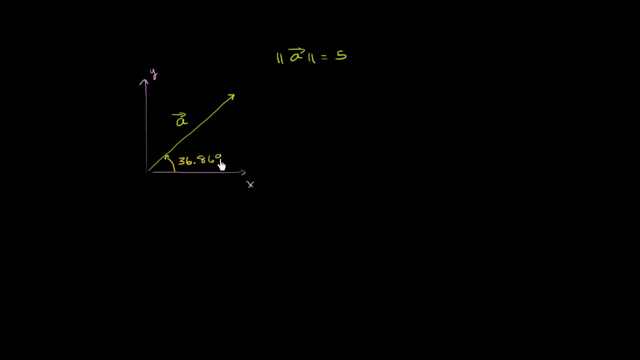 It's 36.8699 degrees. So I'm picking that particular number for a particular reason, And what I want to do is I want to figure out this vector's horizontal and vertical components. So I want to break it down into something that's going straight up or down. 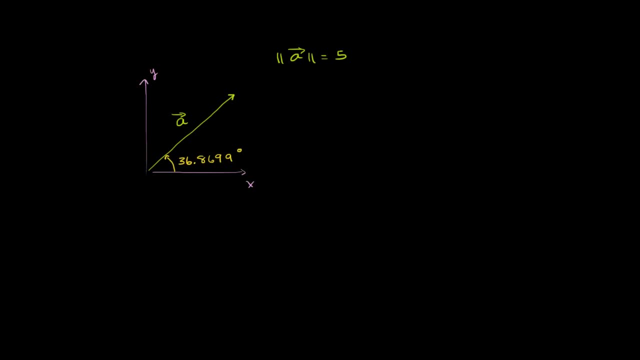 and something that's going straight, right or left. So how do I do this? Well, one, I could just draw them visually see what they look like. So its vertical component would look like this: So it would start. its vertical component would look like this: 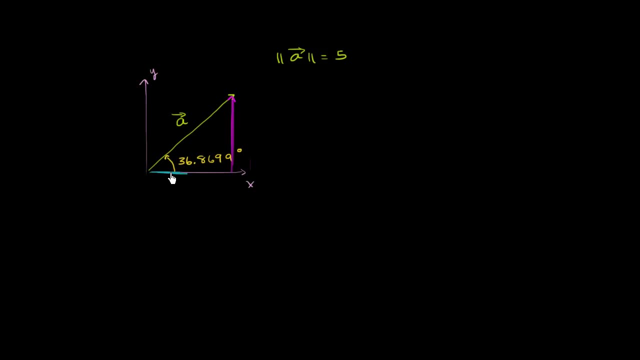 and its horizontal component would look like this. Its horizontal component would look like this. The horizontal component: the way I drew it, would start where vector a starts and go as far in the x direction as vector a starts. So vector a's tip, but only in the x direction. 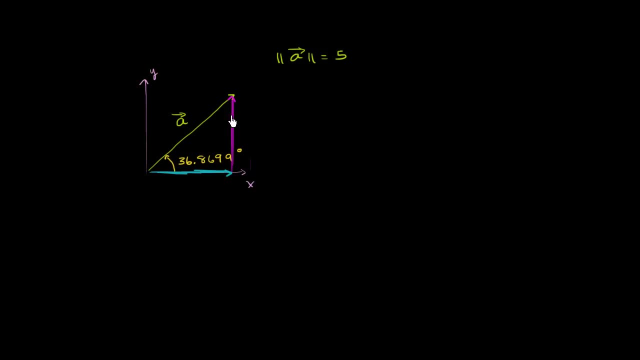 And then to get back to the head of vector a, you need to have its vertical component, And we can sometimes call this: we could call the vertical component over here a sub y, just so that it's moving in the y direction. 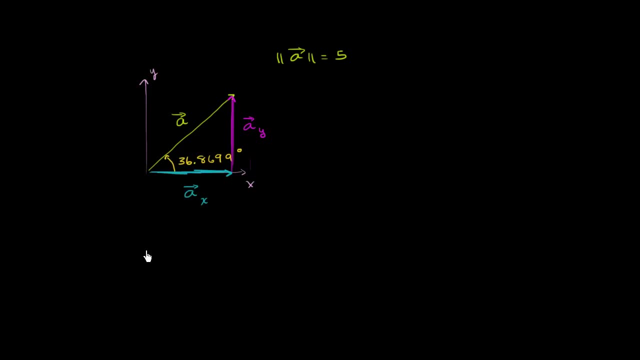 And we could call this horizontal component a sub x. And what I want to do is I want to figure out the magnitude of a sub y and a sub x. So how do we do that? Well, the way we drew this, I've essentially set up a right triangle for us. 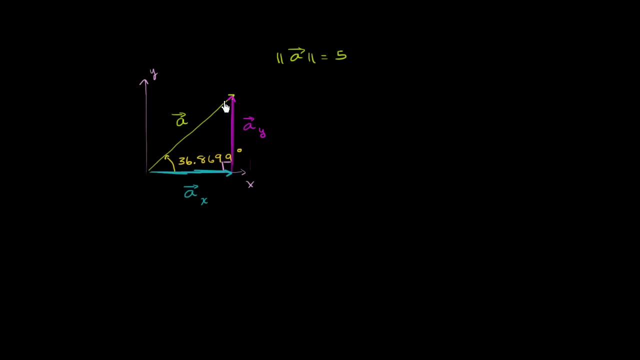 This is a right triangle. We know the length of this triangle, or the length of this side, or the length of the hypotenuse. That's going to be the magnitude of vector a, And so the magnitude of vector a is equal to 5.. 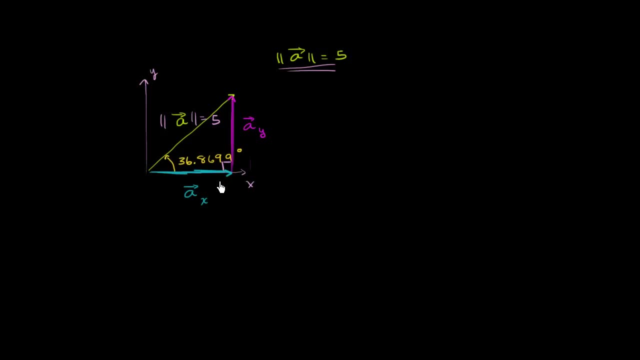 We already knew that up here. So how do we figure out these sides? Well, we could use a little bit of basic trigonometry. If we know the angle and we know the hypotenuse, how do we figure out the opposite side to the angle? 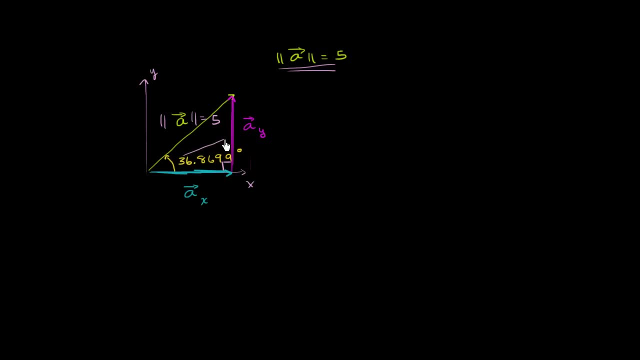 So this right here, this right here, is the opposite side to the angle, And if we forgot some of our basic trigonometry, we can relearn it right now. SOH CAH, TOA Sine is opposite over hypotenuse. 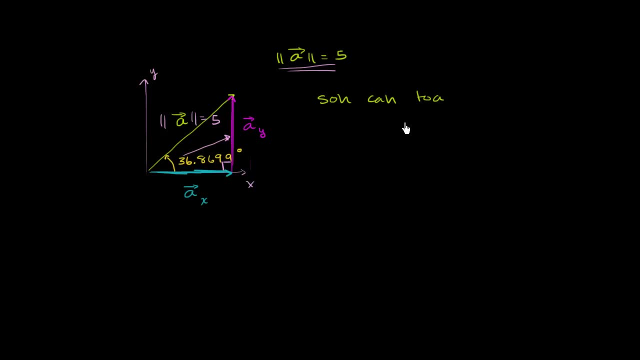 Cosine is adjacent over hypotenuse, Tangent is opposite over adjacent. So we have the angle, We want the opposite and we have the hypotenuse. So we could say that the sine, the sine of our angle, the sine of 36.899 degrees, 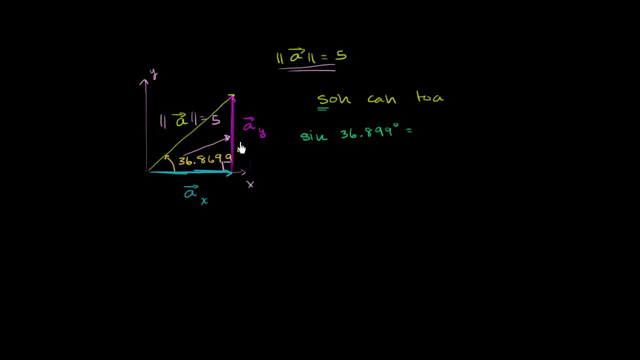 is going to be equal to the opposite over the hypotenuse. The opposite side of the angle is the magnitude of our y component. It's going to be equal to the magnitude of our y component. the magnitude of our y component over the magnitude of the hypotenuse. 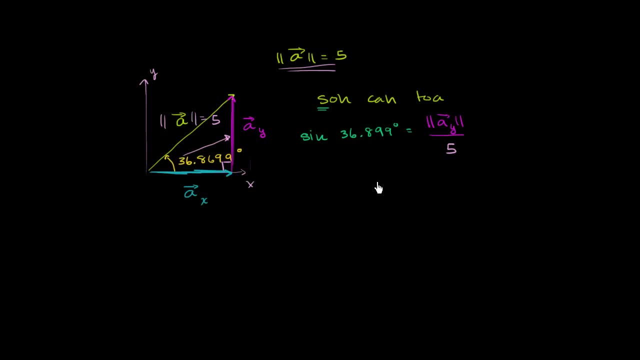 over this length over here, which we know is going to be equal to 5.. Or if you multiply both sides by 5, you get 5 sine of 36.899 degrees is equal to the magnitude, is equal to the vertical component. 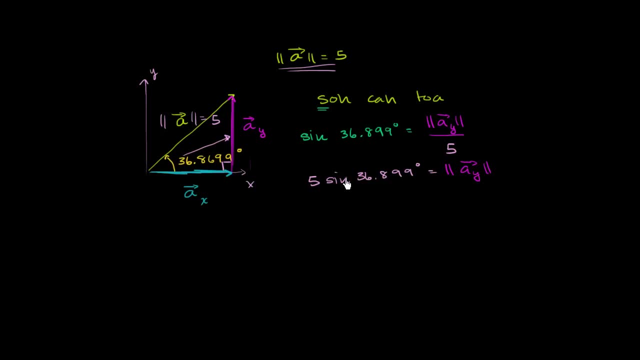 the magnitude of the vertical component of our vector A. Now, before I take out the calculator and figure out what this is, let me do the same thing for the, for the horizontal component. Over here we know this side is adjacent to the angle. 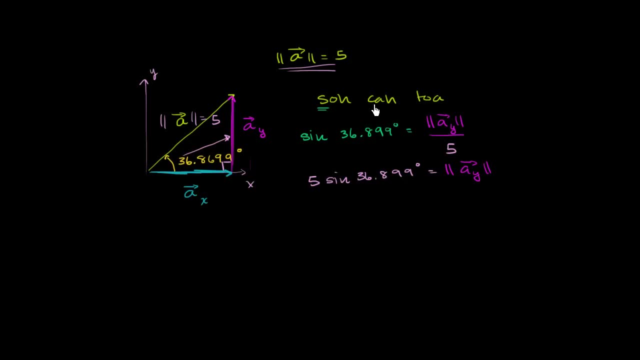 and we know the hypotenuse, And so cosine deals with adjacent and hypotenuse. So we know that the cosine of 36.899 degrees is equal to. cosine is adjacent over hypotenuse is equal to the magnitude of our x. 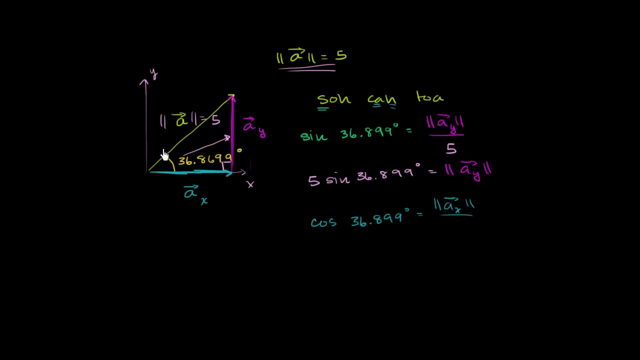 of our x component over the hypotenuse. The hypotenuse here has, or the magnitude of the hypotenuse, I should say, which has a length of 5.. Once again, we multiply both sides by 5, and we get 5 times the cosine. 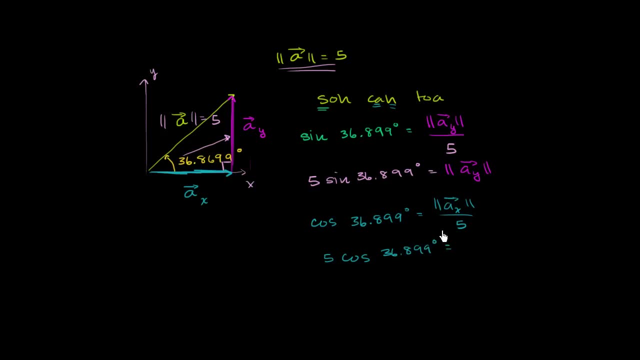 of 36.899 degrees. 36.899 degrees is equal to the magnitude of our x, of our x component. So let's figure out what these are. Let me get the calculator out, Let me get the, let me get my trusty TI-85 out. 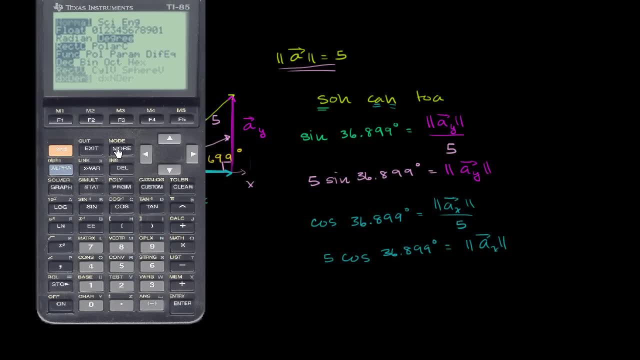 I want to make sure it's in degree mode. So let me check. Yep, we're in degree mode right over there. Don't want to make sure we're not in radian mode. Now let's exit that And we have. the vertical component is equal to. 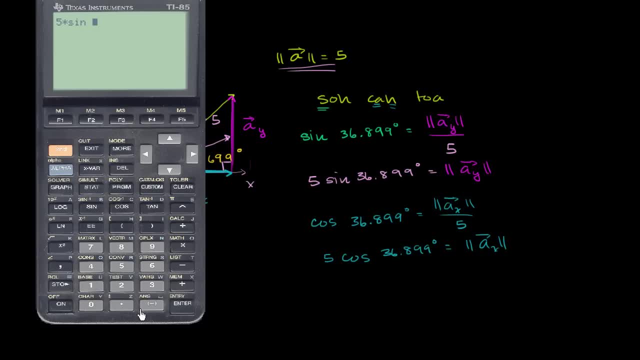 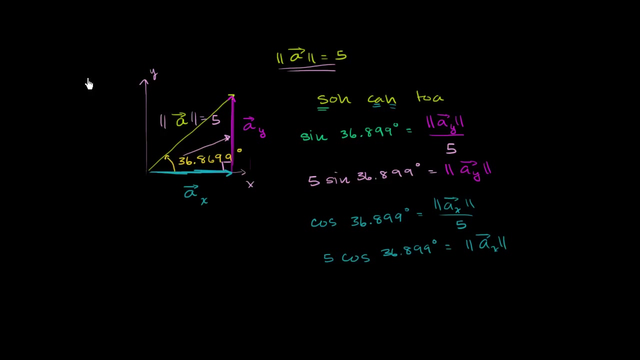 5 times the sine, the sine of 36.899 degrees, Which is, if we round it right, at about 3.. So this is equal to. so the magnitude of our vertical component is equal to 3, is equal to 3.. 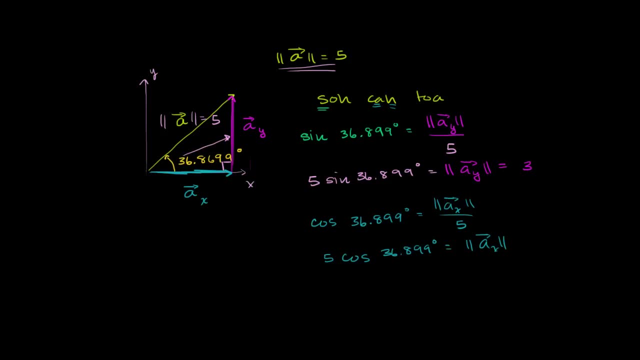 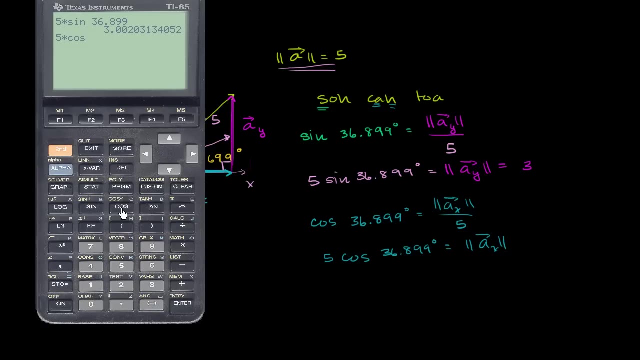 And then let's do the same thing for our horizontal component, For our horizontal component. So now we have 5 times, 5 times the cosine of 36.899 degrees Is if we once again, if we round it to. 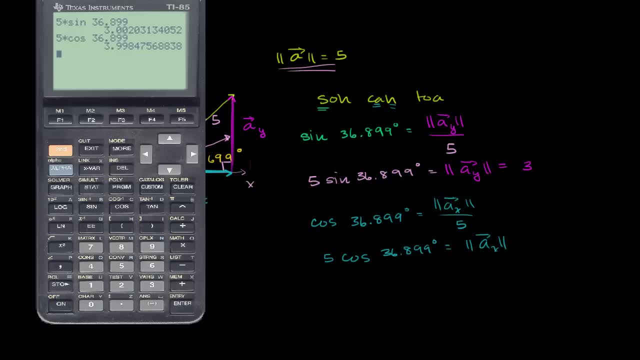 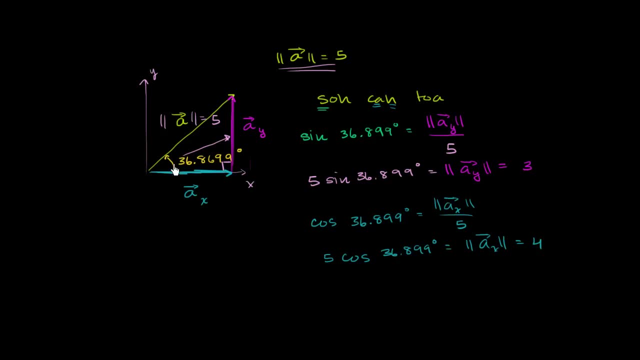 I guess, our hundredths place. we get it to being 4.. So we get it to being 4.. So what we see here is a situation where we have- this is a classic 3-4-5 Pythagorean triangle. 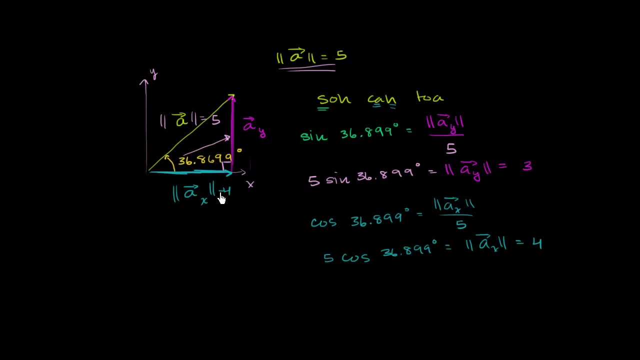 The magnitude of our horizontal component is 4.. The magnitude of our vertical component, the magnitude of our vertical component right over here, is equal to 3.. And once again you might say, Sal, you know why are we going through all of this trouble?